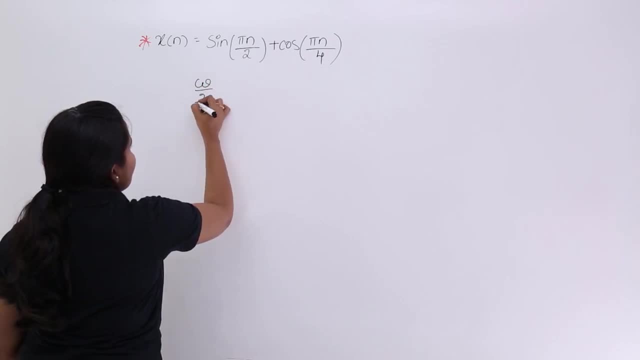 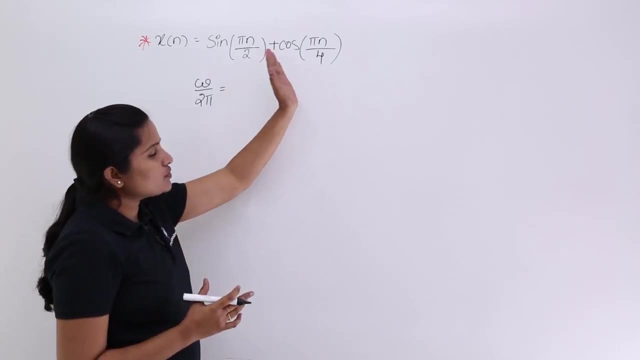 calculate periodicity is omega by 2 pi. If this is rational number then you can say that is periodic, otherwise aperiodic. Here, whenever two signals or combination of signal is given, the resultant signal is periodic, whenever the Periods. here. that means here you are used to calculate n 1 or here you are used to calculate 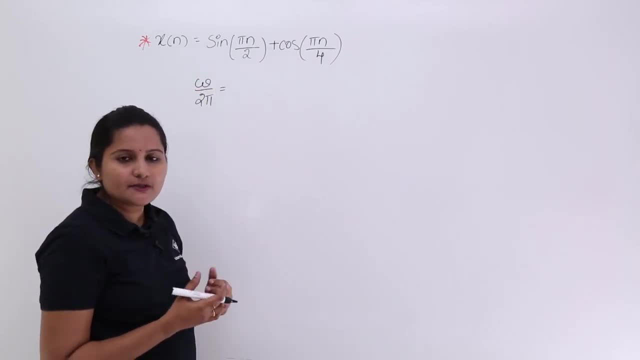 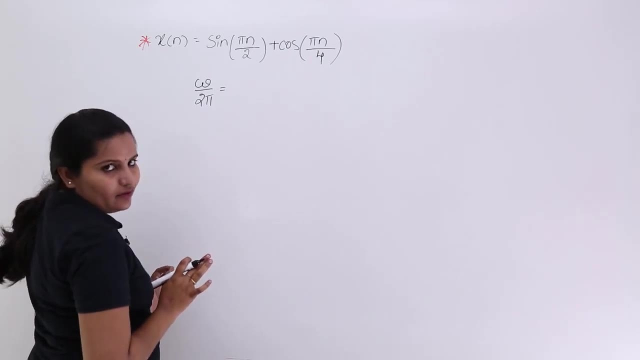 n 2. The LCM of n 1 and n 2 is possible. then you can say that is periodic. So here I want to calculate first of all n 1 for that. So here I need omega 1 by 2 pi value. So I want: 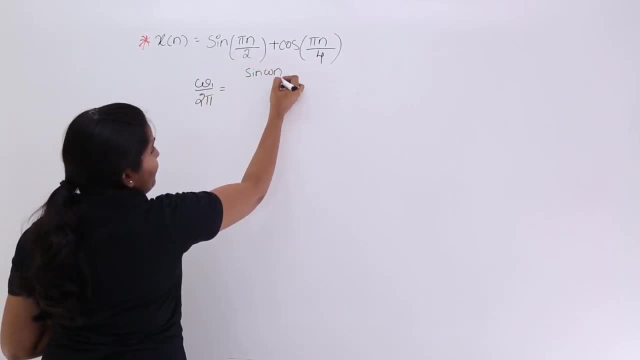 to compare with sin omega n by omega n. I want to compare with the standard equation of sin omega n, and so it is sin omega n. If I compare with sin omega n, my omega value will be pi by 2.. So divided by 2 pi. So here this is equal n 2. So pi by 2 by 2 pi means pi, pi. 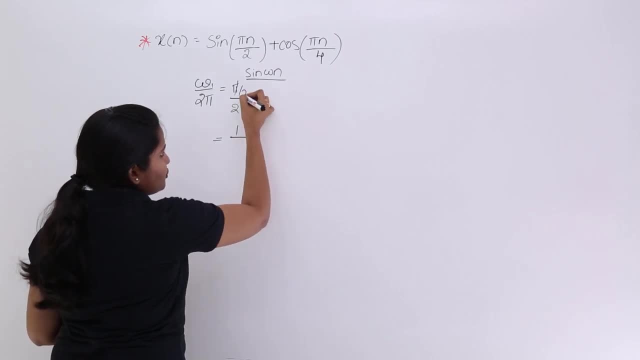 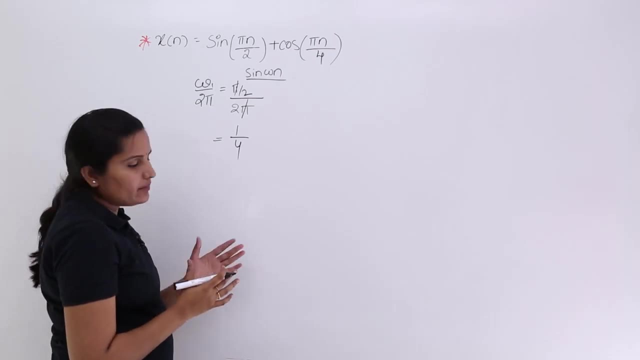 will gets cancelled and divided by 2 will come to denominator. So 1 by 4 will come. So this is a periodic signal. because up to here this is a periodic signal why? because So you are having integer by integer format for this ratio. So this is equivalent to: 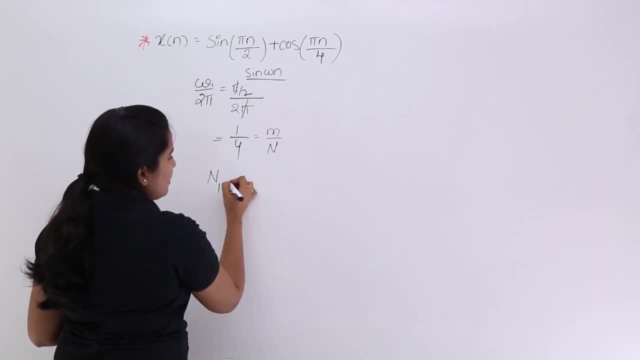 m by capital N, where N is equivalent to number of sample For this signal, the number of samples is equivalent to 4. that means one full cycle you require. N is equivalent to 4 samples. So here now I am going to consider another value. So another value, that means another. 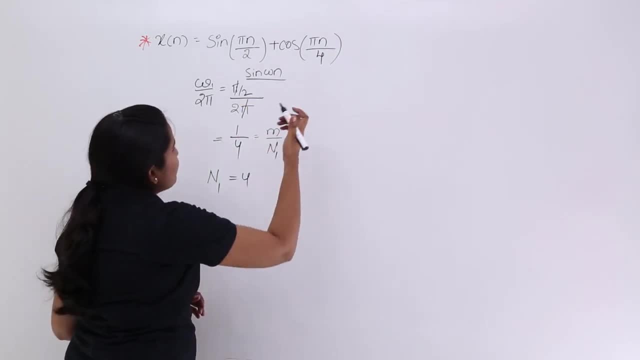 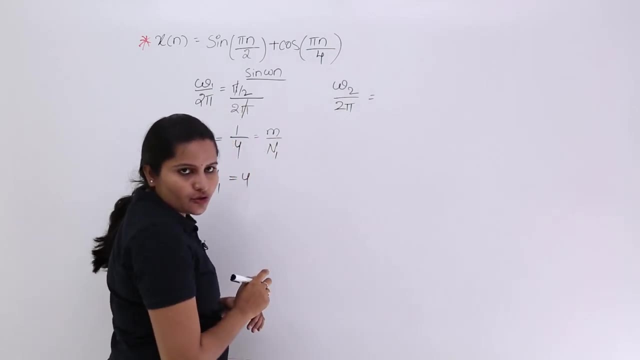 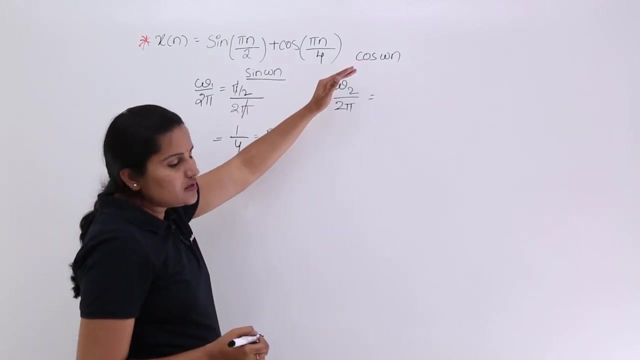 period of next part of the signal. Speaker 1. So here also I want to calculate omega 2, pi 2, pi, So to trace the value of omega 2, I am going to compare with cos omega n. this is the standard cos signal. So discrete cos, So cos omega n. if 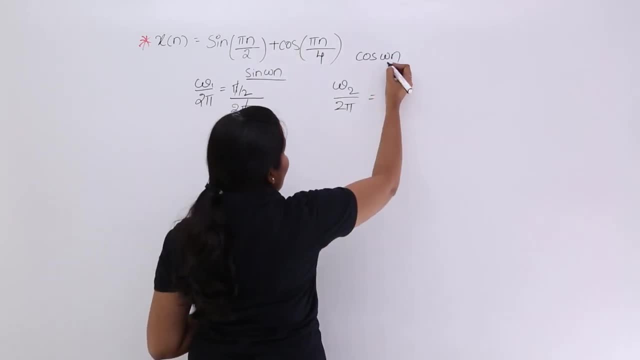 you compare your omega n or omega value will be pi by 4 divided by 2. pi, you are going to consider pi. pi gets cancelled, So this will be equivalent to 1 by 8. you are going to get 8 here. So now,